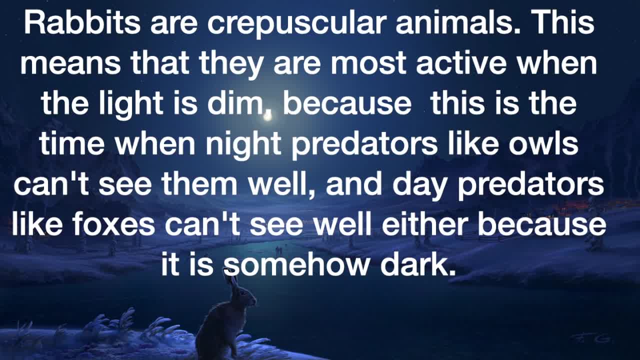 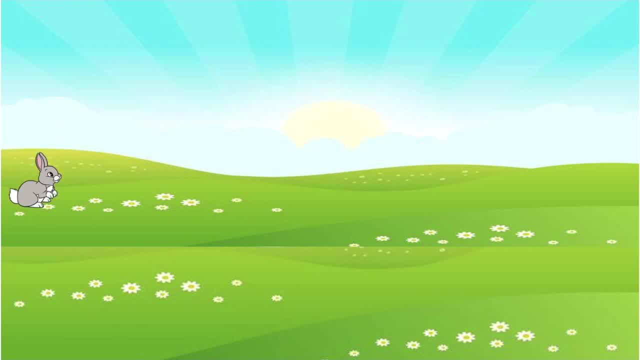 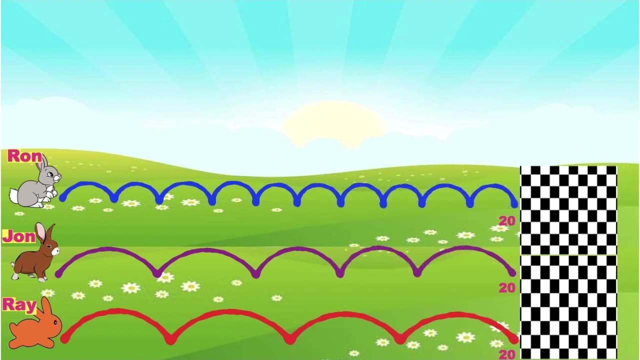 like foxes, can't see well either because it is somehow dark. I have here three rabbits Name Ron, John And Ray. These three rabbits joined a rabbit hopping competition. Based on the given pictures, who do you think will reach 21st? 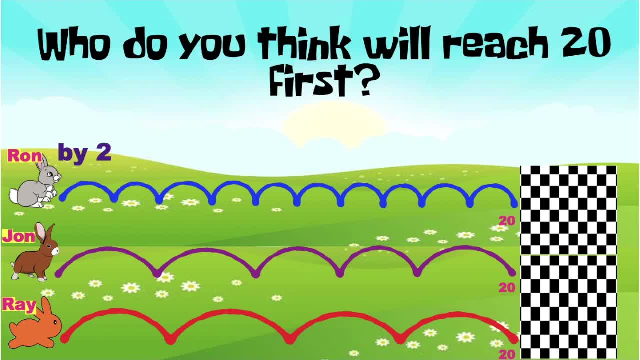 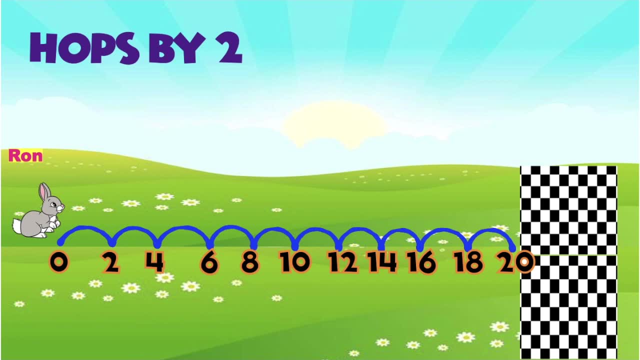 If Ron will hop by two, if John will hop by four and if Ray will hop by five. Let's have a closer look at the rabbit hopping contest. Let's see who Ron hops by. Ron hops by two, Two, four, six, eight, ten, twelve, fourteen, sixteen, eighteen, twenty. 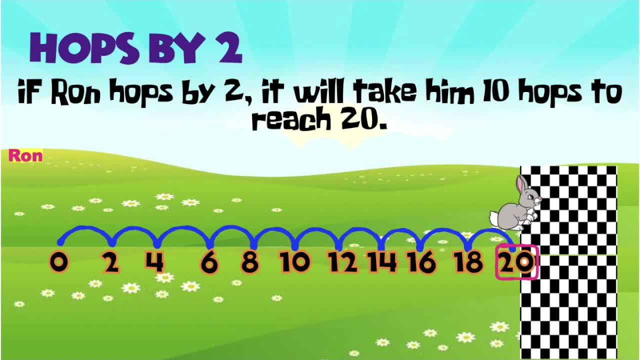 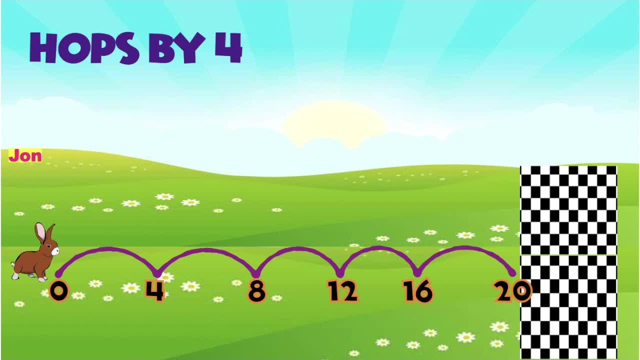 If Ron hops by two, it will take him ten hops to reach twenty. You're on your way. Let's look now at Jon. Jon hops by four, Four, eight, twelve, sixteen, twenty. If Jon hops by four, it will take him five hops to reach twenty. 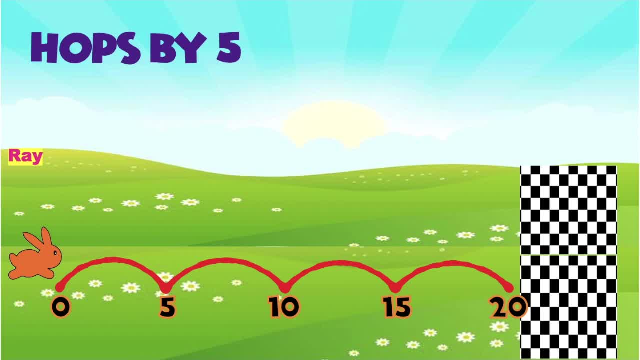 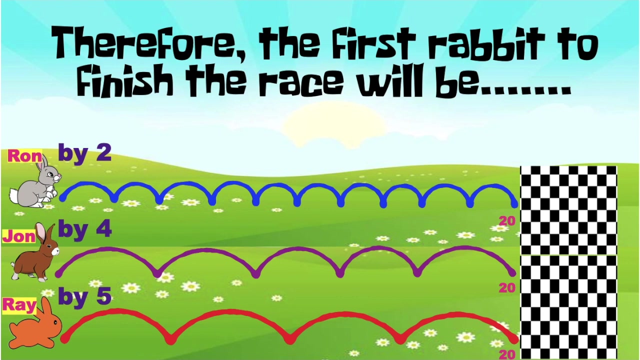 Let's proceed to Ray. Ray hops by five, 5,, 10,, 15,, 20.. If Ray hops by 5, it will take him 4 hops to reach 20.. Therefore, the first rabbit to finish the race will be: 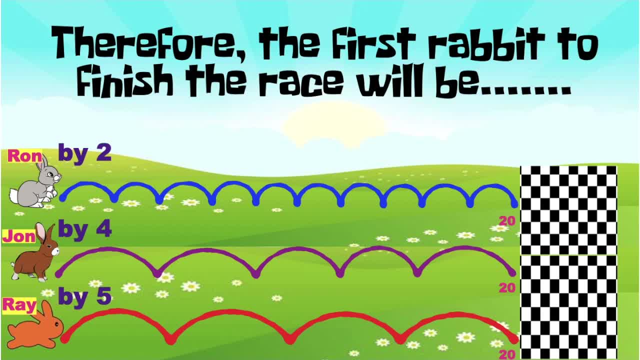 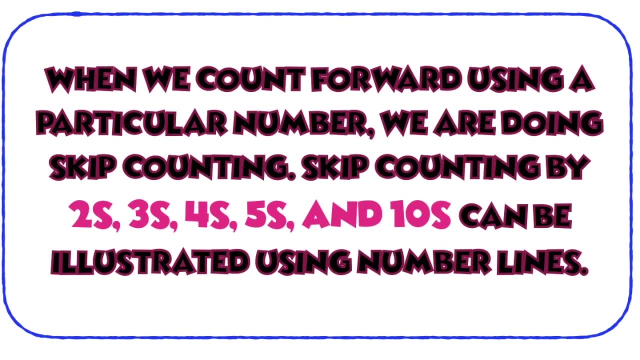 That's correct, It's Ray. So when we count forward using a particular number, we are doing skip counting. Skip counting by 2s, 3s, 4s, 5s and 10s can be illustrated using number lines. 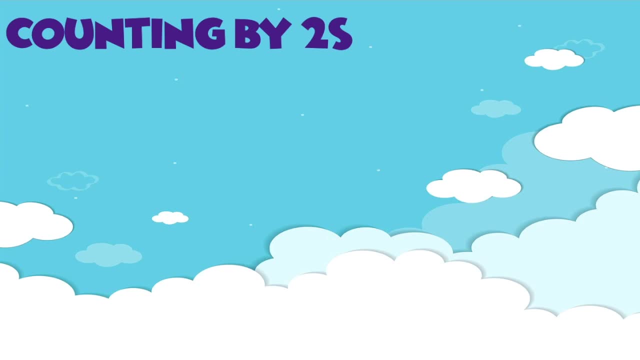 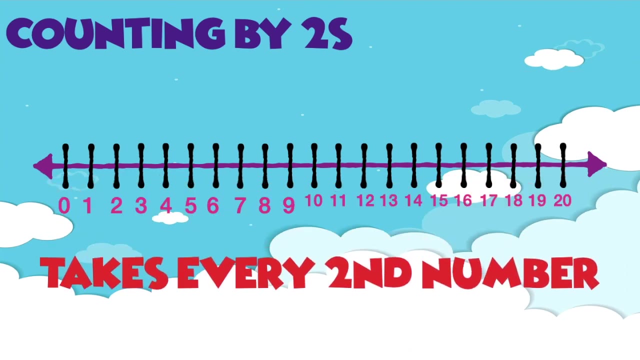 Let's have skip counting by 2s using this number line. When you say skip counting by 2s, it takes every second number. Also, we add 2 after every number. So let's start at 0, going to 2.. 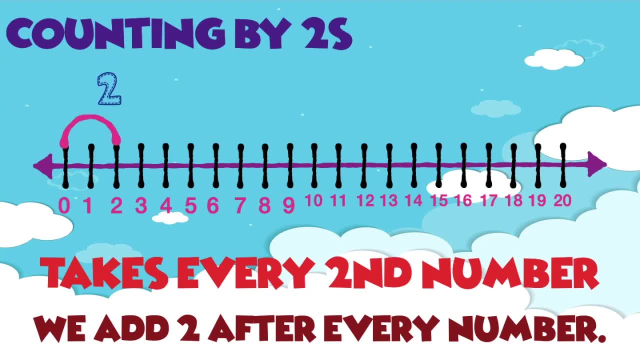 2,, 4,, 6,, 8,, 10,, 12,, 14,, 16,, 18,, 20.. So this is skip counting by 2s. Again, children always remember when you say: skip counting by 2s. 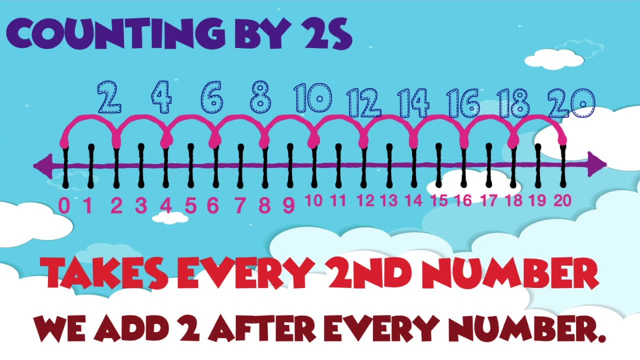 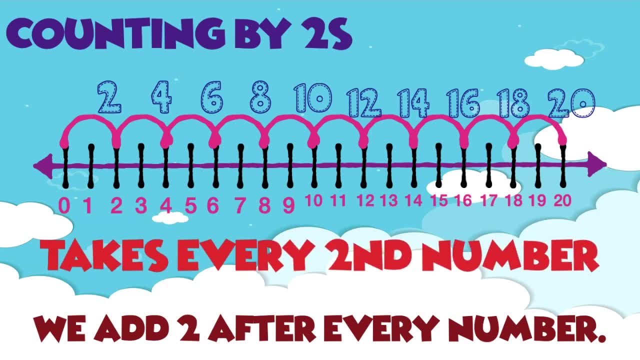 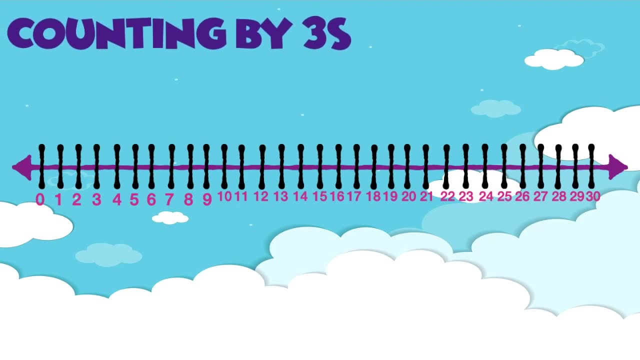 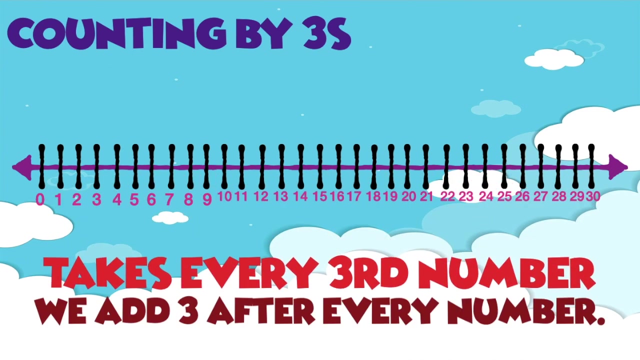 it takes every second number. Also, we add 2 after every number. So let's have skip counting by 3s. Again, in skip counting by 3s it takes every third number And we add 3 after every number. 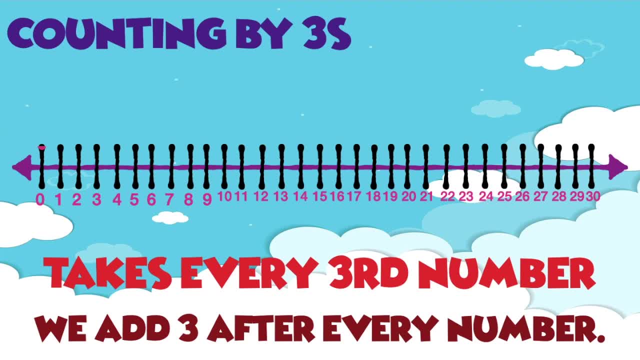 So let's start at 0, going to 3., 3., 3., 3., 6., 6., 9., 9., 12., 12., 15., 15., 18., 18.. 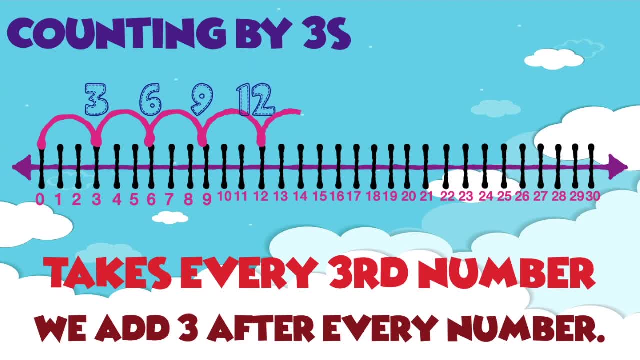 21., 21., 24., 24., 24., 25., 25., 26., 26., 27., 27., 28., 29., 29., 30., 30., 31.. 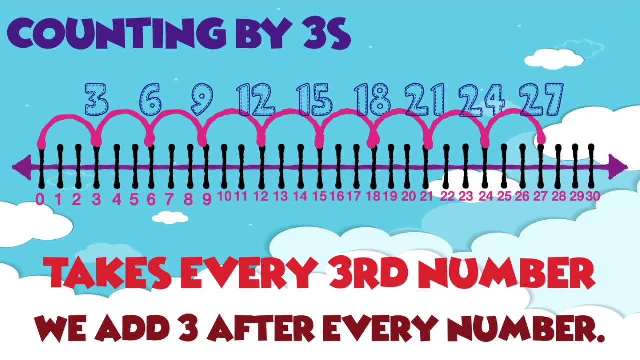 31., 32., 27., 27., 30. So this is skip counting by 3s. Again, it takes every third number. Also, we add 3 after every number, So let's have skip counting by 4s. 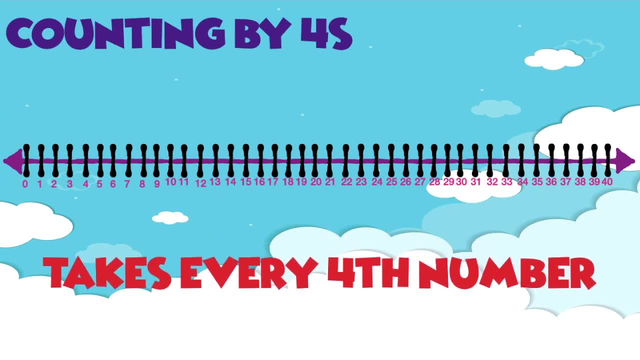 In skip counting by 4s, it takes every fourth number And in able to find the next number, you need to add 4. After every number. So let's start at 0, going to 4. 4. 4.. 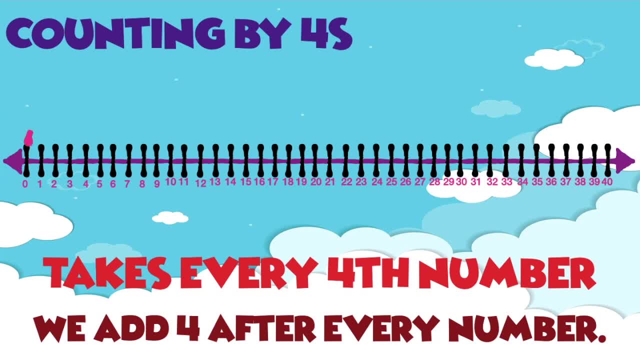 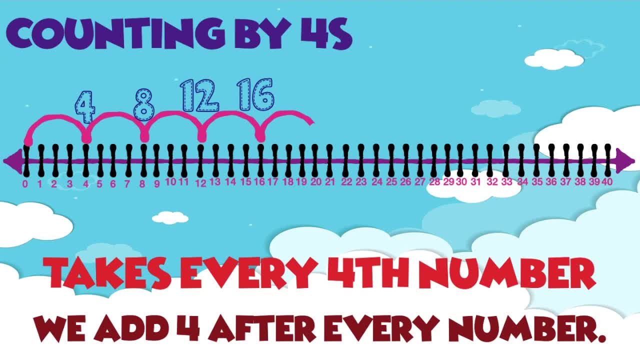 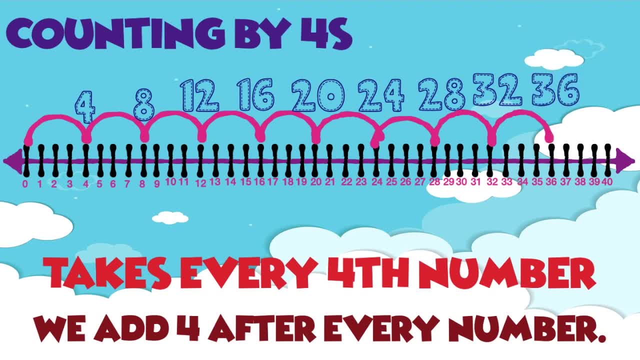 17., 17., 18., 19., 20., 21., 22., 23., 34., 24., 25., 28., 32., 36., 40., 35. So this is skip counting by 4s. 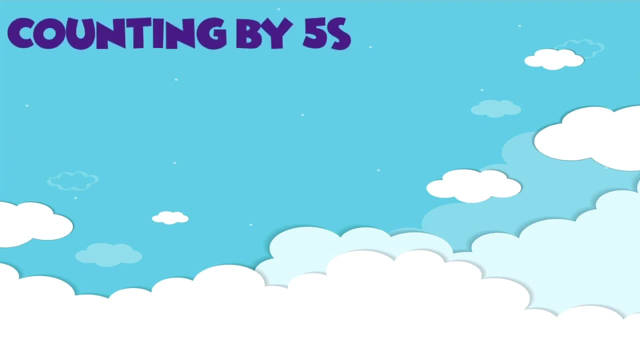 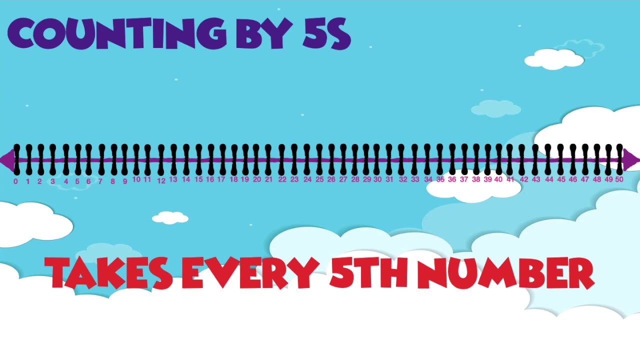 Again: children: in skip counting by 4s it takes every fourth number Also. we add 4 after every number. now to skip counting by fives. in skip counting by fives it takes every fifth number also. we add five after every number. five count with me. children, five, ten, fifteen. 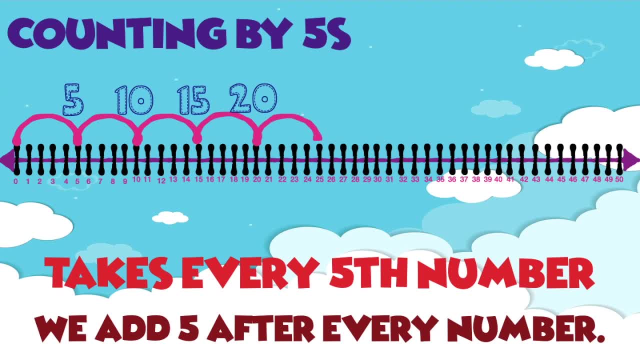 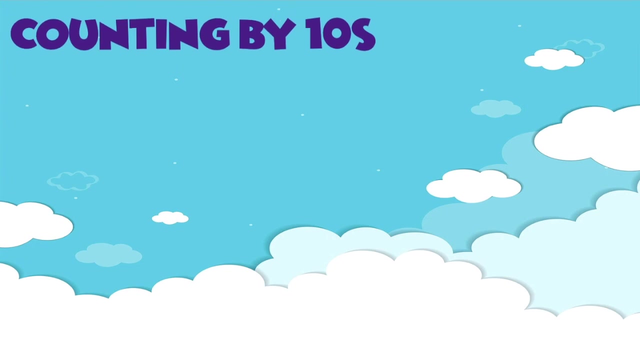 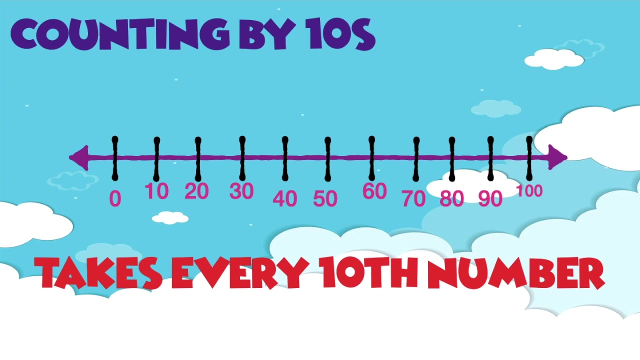 twenty, twenty five, thirty, thirty five, forty, forty five and fifty. so this is skip counting by fives. again, in skip counting by fives it takes every fifth number also. we add five after every number. so let's go now to skip counting by tens. so in skip counting by tens, it takes every tenth number also. we add 10 after every number. 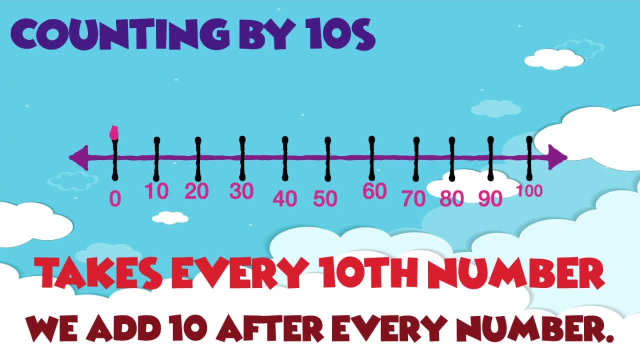 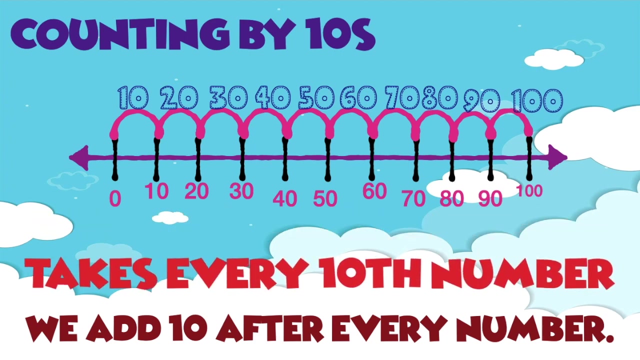 so let's start count with me children: 10, 20, 30, 40, 50, 60, 70, 80, 90 and one hundred. so this is keep counting by tens. again, in skip counting by tens, it takes every 10 number and we add 10 after every number. 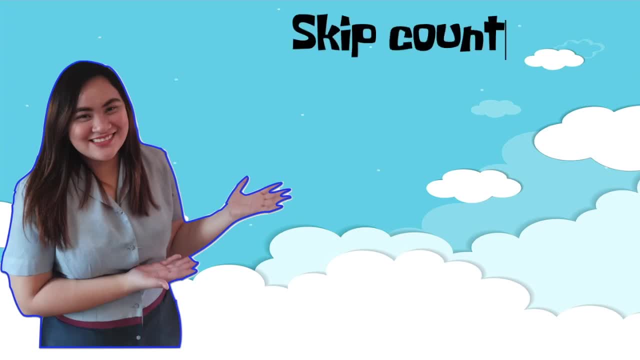 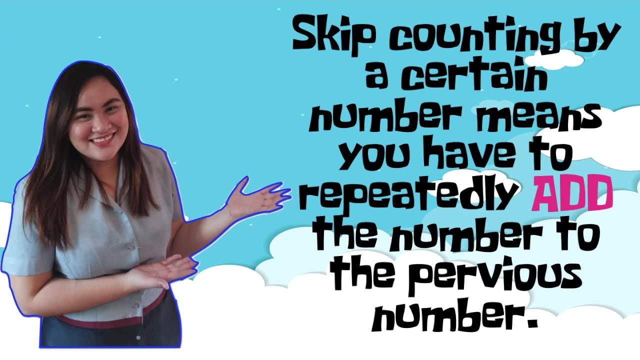 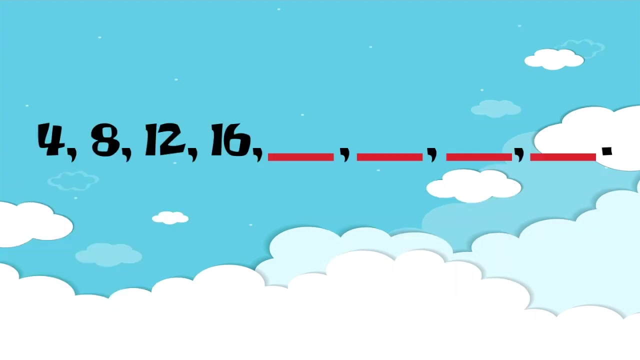 Skip counting by certain number means you have to repeatedly add the number to the previous number. So I have here the set of numbers and I want you to find the skip counting that we're going to use in able to find the missing numbers, For us to find what kind of skip counting are we going to use here is we're going to count forward from 4 until we reach 8. 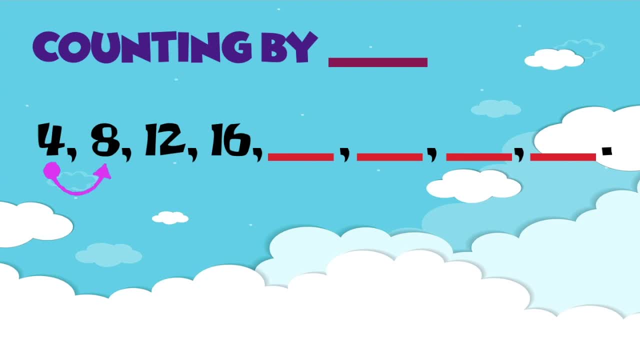 So, using your fingers, children, let's count from 4 until we reach 8. 4 on your mind. 4, 5, 6, 7, 8. So that means Digit 8 is the fourth number from 4. That's why we're going to use skip counting by fourth. 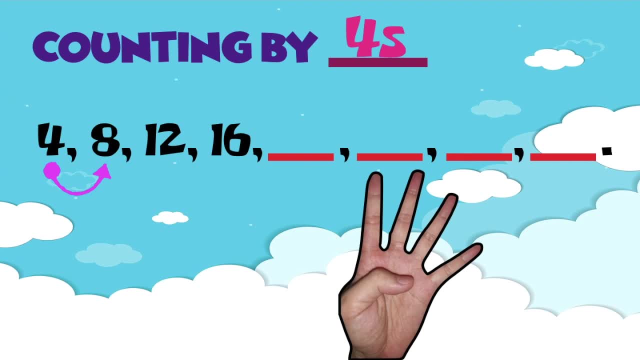 So now, we can now start finding the missing numbers. So from 16, We're going to count forward until we reach the fourth number. So 16 on your mind, 16, 17, 18, 19, 20. So the next number is 20. So from 20, 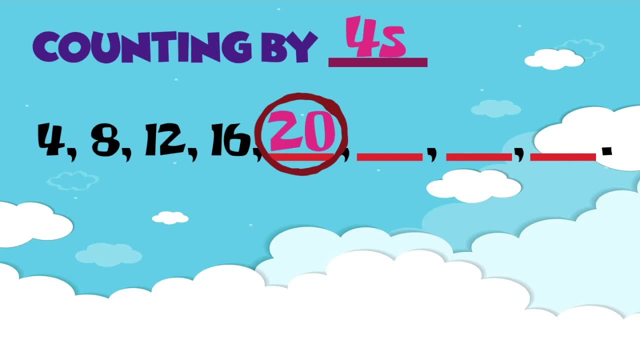 Let's count again to find the fourth number: 20 on your mind. 20, 21, 22, 23, 24. That means the next number is 20, 24. So from 24 Let's count again the fourth number, So 24 on your mind. 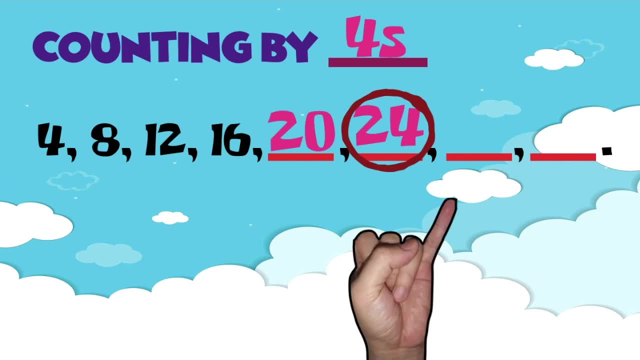 24, 25, 26, 27, 28, So the next number is 28. So now let's have 28, 28 on your mind, 28, 29, 30, 31, 32, So the last number is 32. So this is skip counting by fourth. 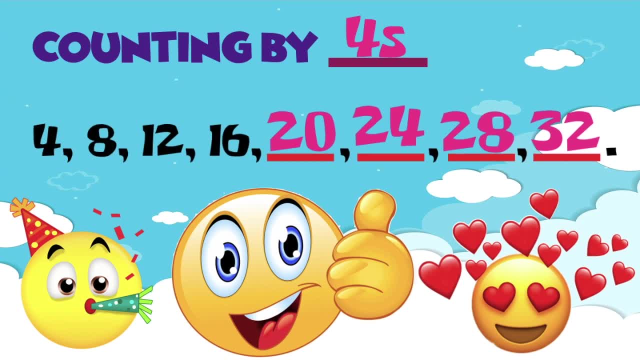 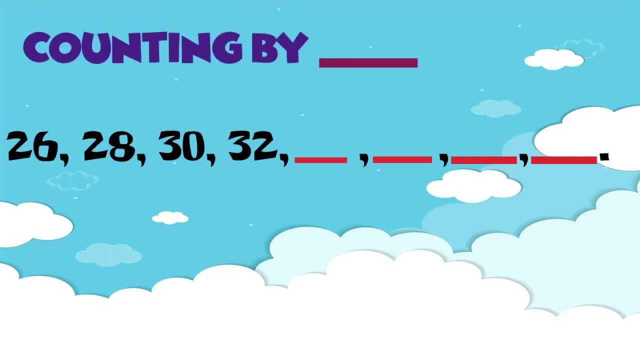 How about, if we have this? Let's find again what kind of skip counting are we going to use. So again, children, in able to find what kind of skip counting you're going to use, You need to count forward From the first number. So let's count from 26 until we reach 28. 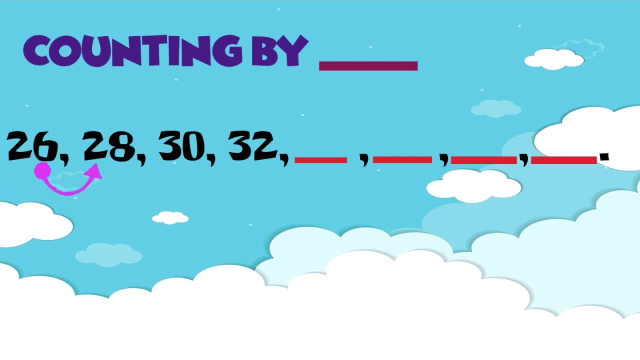 Clear. So 26 on your mind, 26, 27, 28. So this is skip counting by twos, Because 28 is the second number from 26. So now we're ready to find the missing numbers. So let's start at 32. So 32 on your mind. 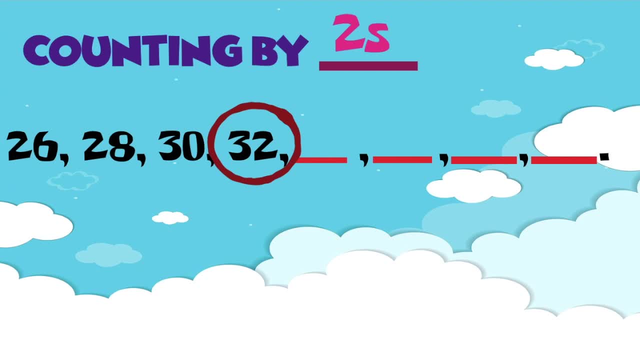 32. let's count using your fingers: 32, 33, 34. So the next number is 34, Because it is the second number After 32. Okay, so let's find the second number from 34, So 34 on your mind, 34, 35. 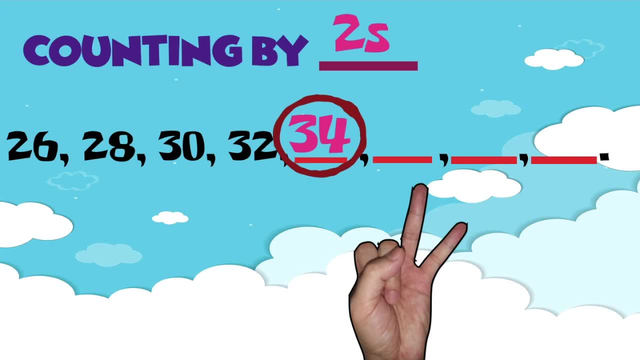 36, So the next number is 36. Okay, from 36 let's count again: 36 on your mind, 36, 37, 38, So we have 38. So now children: 38 on your mind, 38, 39, 40, So we have 40 here. 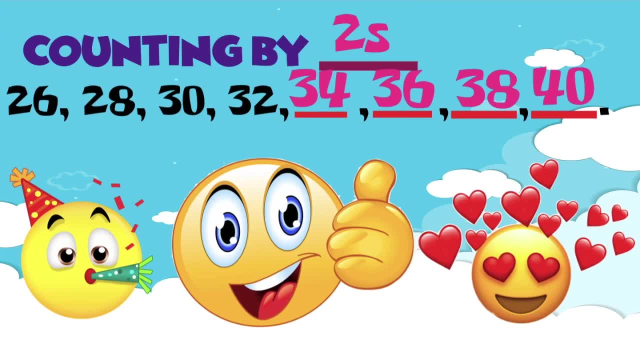 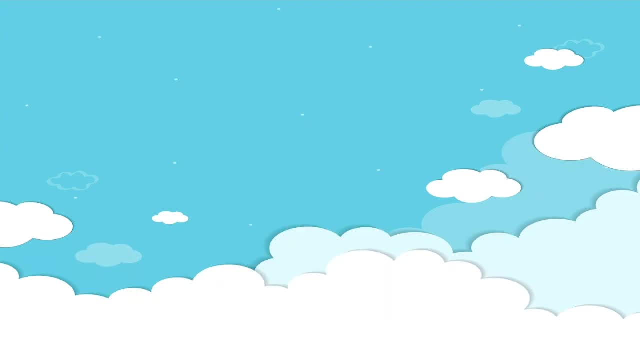 So this is skip counting by twos. Let's have the next number. How about, if we have this? Let's find again what skip counting is. Are we going to use in able to find the missing numbers? So let's start at 60 until we reach 65. 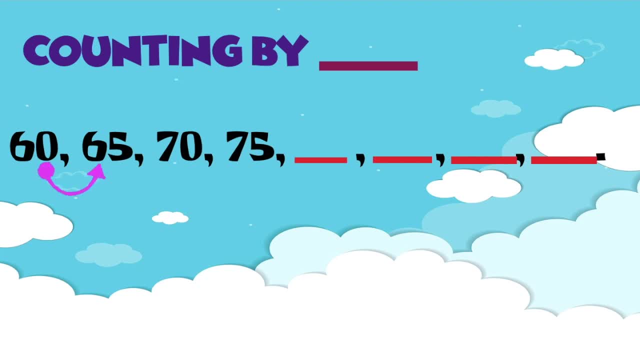 So, 60 on your mind, children, Let's count using your fingers. 60 on your mind. 60, 61, 62, 63, 64, 65. So we have skip counting by fives, Because the number 65 is the fifth number from 60. That's why we're going to use skip counting by fives. 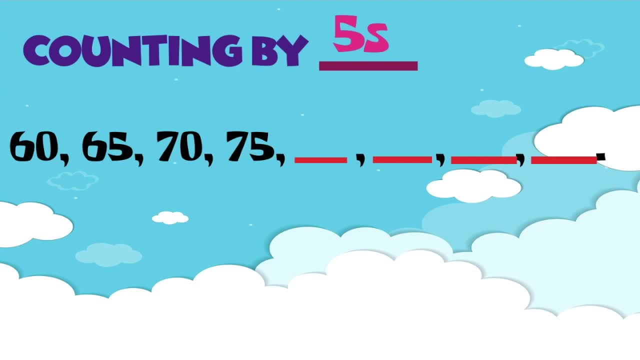 So now let's find the missing number. Let's start counting from 75 So 75 on your mind. 75, 76, 77, 78, 79, 80. So we have 80. So now let's have the next number, 80, on your mind. 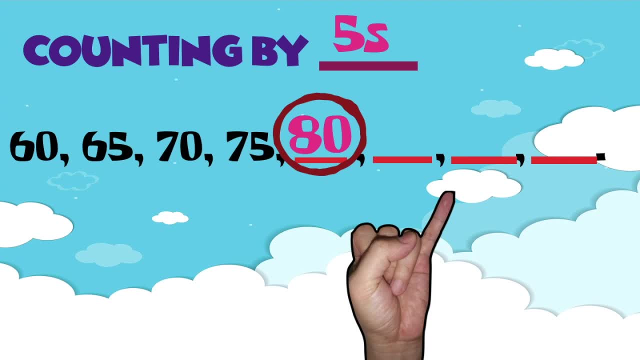 80, 81, 82, 83, 84 And 85, So we have 85 here. So, okay, let's have the next number- 85 on your mind. 85, 86, 87, 88, 89, 90, So we have 90 here. So let's have the last number. 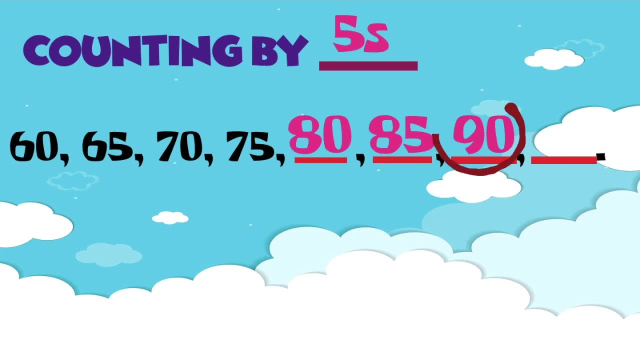 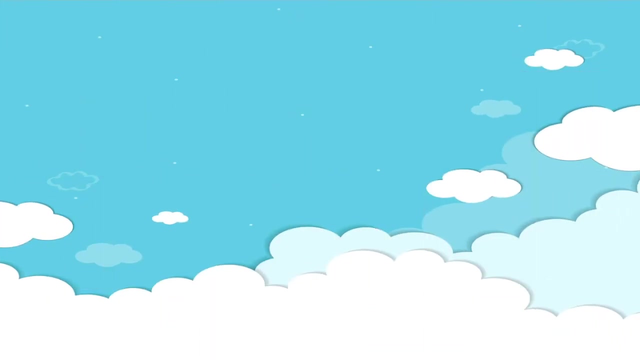 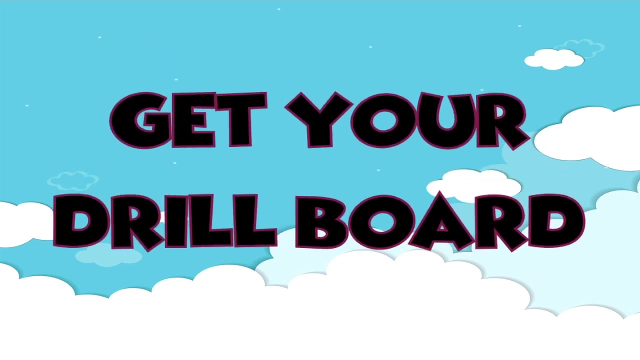 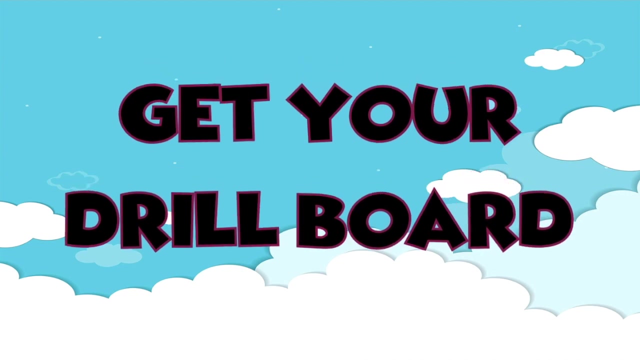 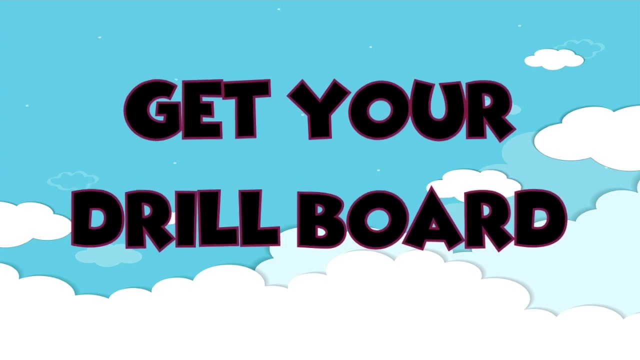 90 on your mind, 90, 91, 92, 93, 94 And 95, So we have here 95. So this is skip counting by fives. Okay, everybody, please get your drill board. So, using your drill board, Let's have this exercise. So I want you to identify the skip counting. 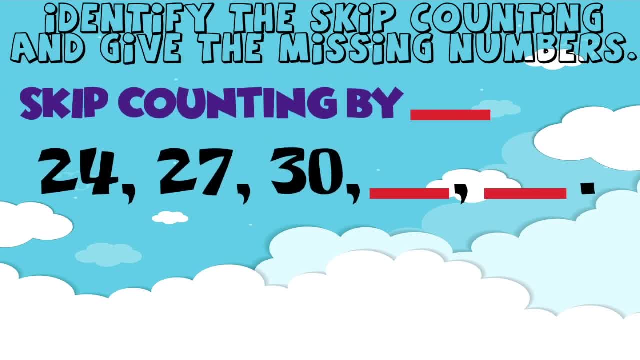 And give the missing numbers. So let's have the first one. Timer starts now. Write your answer on your drill board. You may use your fingers in counting. Write your answer in half a second. Give it a second try. Give your answer a second try And then you can repeat. 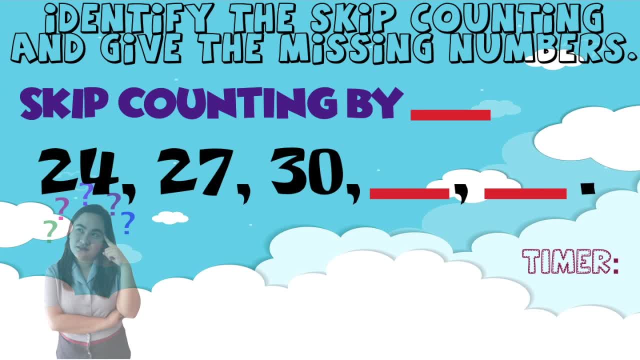 Write and repeat, And repeat, And repeat, Repeat, Repeat, Repeat, Repeat, Repeat And repeat. Time's up. So let's see if your answer is correct. So, for us to find what kind of skip counting are we going to use, We need to count forward from 24 until we reach 27. 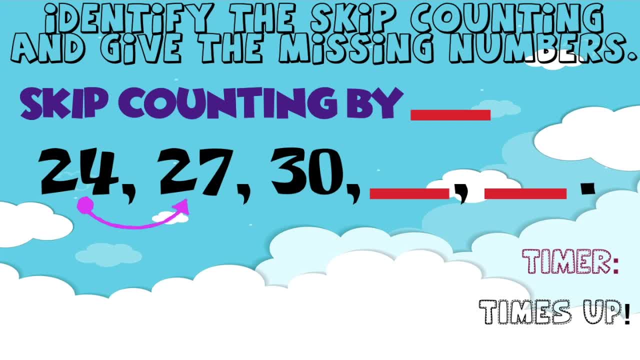 So let's count. So that means from 24, 27 is the third number. That's why we're going to use skip counting by threes. So now let's find the missing numbers. Let's start at 30. 30 on your mind, 30. 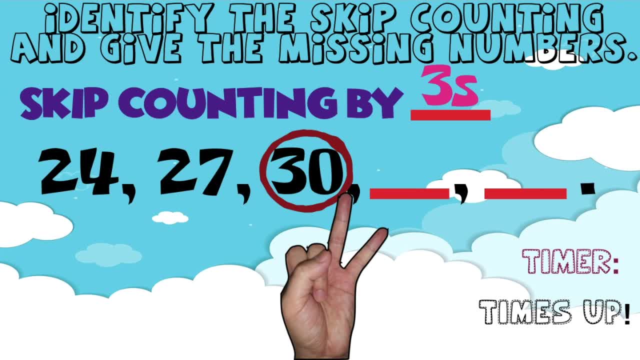 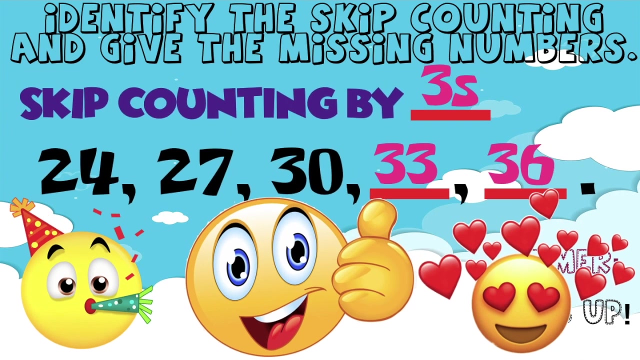 31, 32, 33, So the first missing digit is 33. So now let's find the next missing number. So from 33, 33, on your mind, 33, 34, 35, 36, So we have 36. So that is the answer We have here. skip counting by threes. 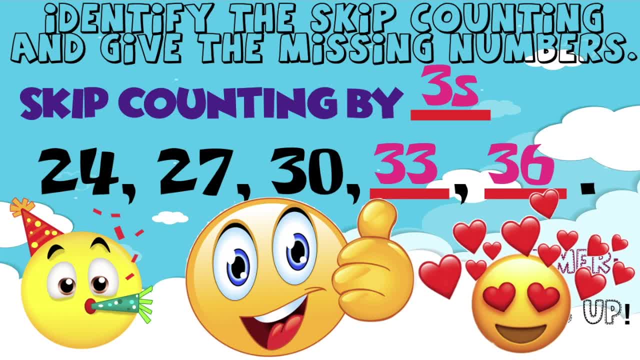 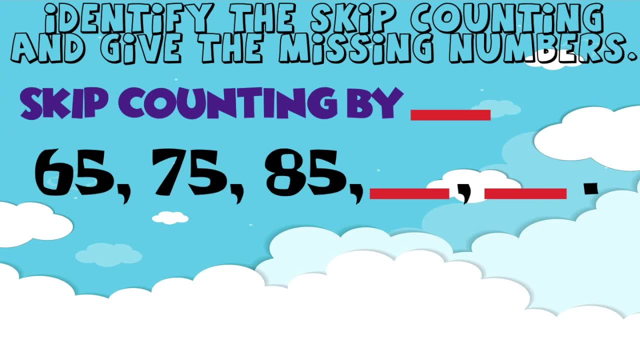 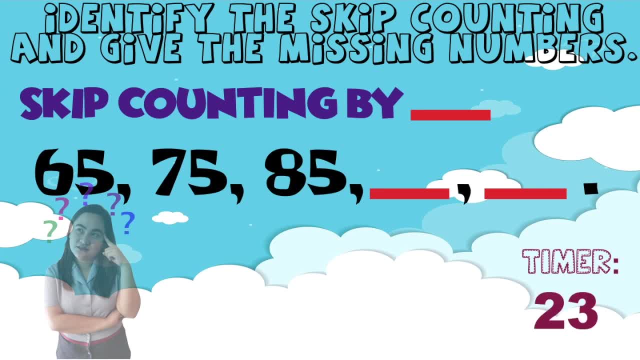 Let's start. Let's start. Thank you, Time's up, So let's see if your answer is correct. So, for us to find what kind of skip counting are we going to use here, let's count from 65 until we reach. So let's use your fingers in counting. 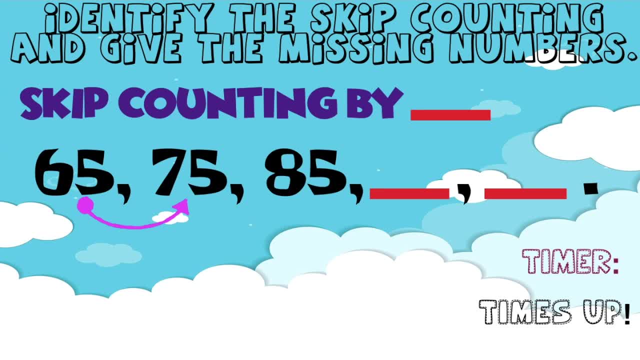 So 65 in your mind, 65, 66,, 67,, 68,, 69,, 70,, 71,, 72,, 73,, 74,, 75. So that means from 65,, 75 is the 10th. 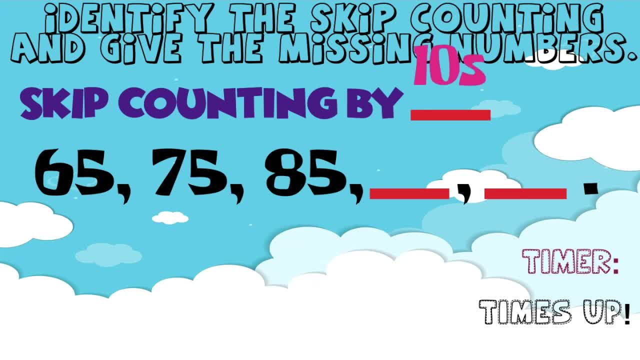 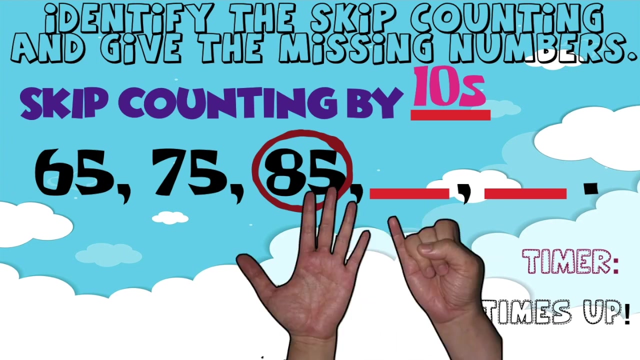 Number. That's why we're going to use skip counting by 10.. So now we're ready to find the missing number, So let's start at 85.. So 85 in your mind: 85, 86, 87, 88, 89, 90,, 91,, 92,, 93,, 94,, 95.. 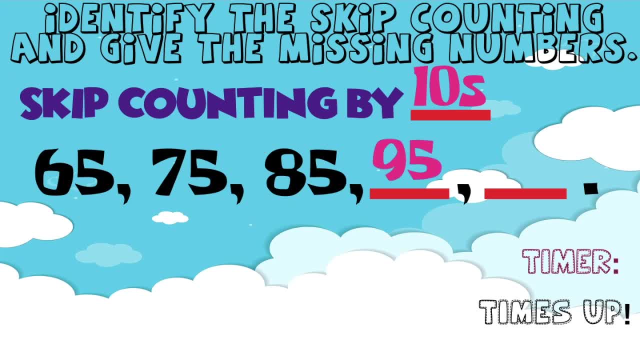 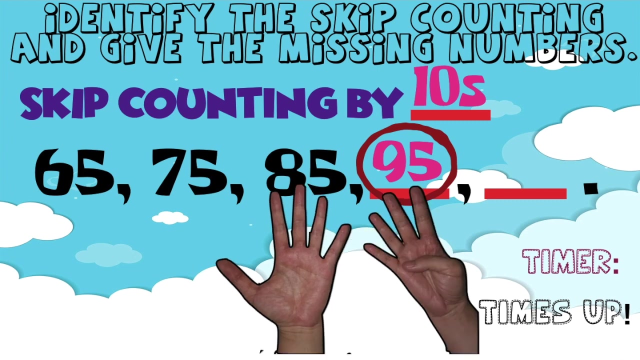 So the next number after 85 is 95.. So now let's proceed to the last number, 95, on your mind. 95, 96, 97,, 98,, 99,, 100,, 101,, 102,, 103,, 104,, 105. 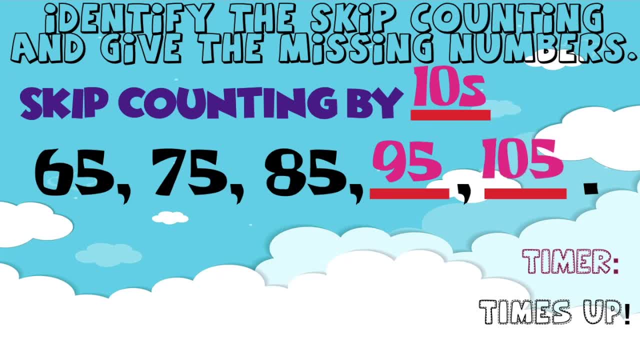 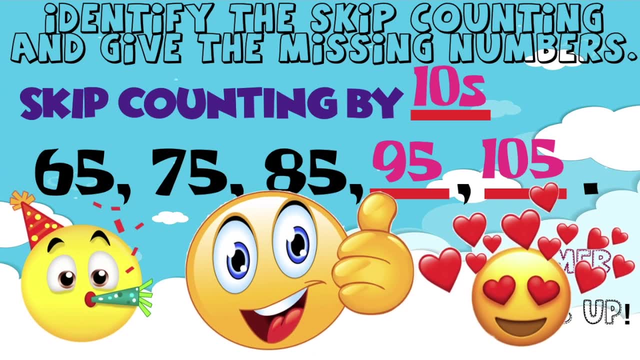 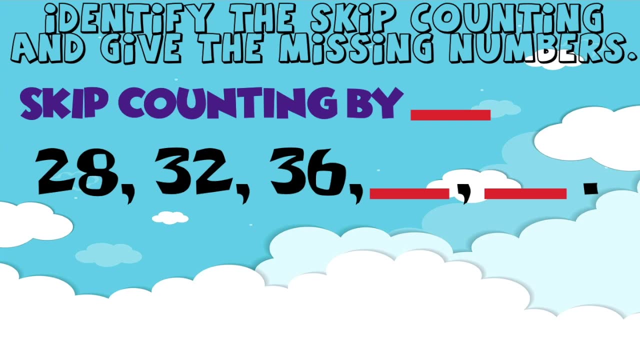 So we have 105. here. so this is keep counting by 10. so let's have the next number. how about if I have this? so timer starts now. you time's up. let's see if your answer is correct. so for us to find the skip counting, let's count. 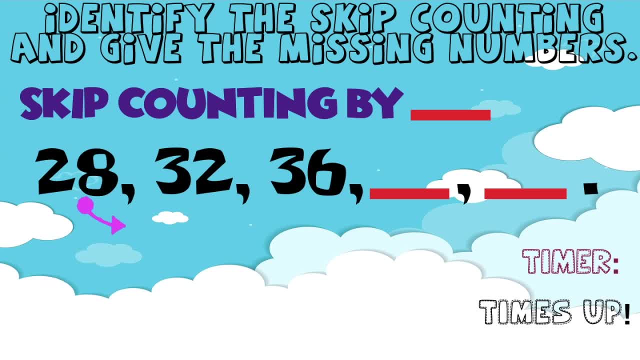 from 28 until we reach 32. 28 on your mind. so let's have the next number: 28, 29, 30, 31, 32. so that means from 28, 32 is the fourth number, so we're going to use skip counting by force. so now let's proceed to 36 until we reach the next number, the fourth. 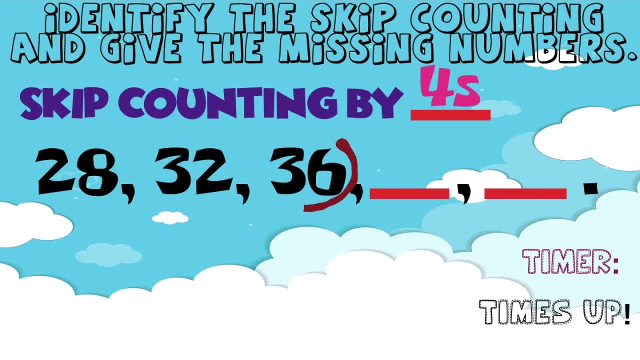 number from 36, so 36 on your mind. let's use your fingers: 36, 36, 37, 38, 39, 40. so the next number is 40. let's have 40, 40 on your mind. 40, 41, 42, 43, 44. so we have. 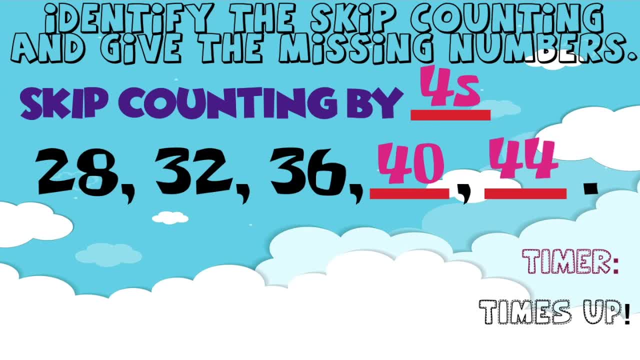 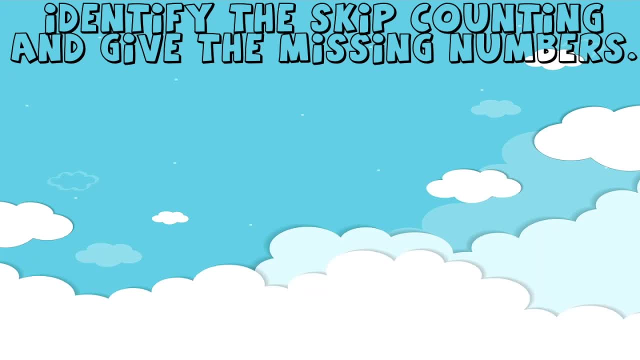 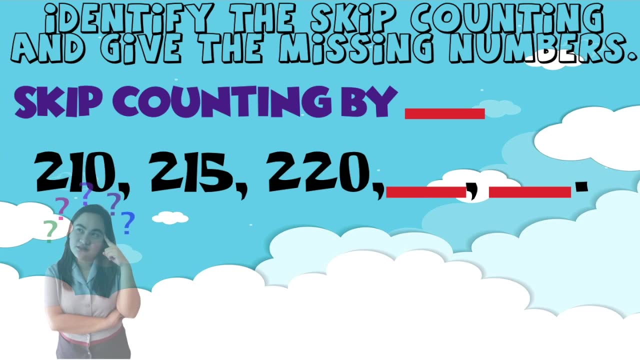 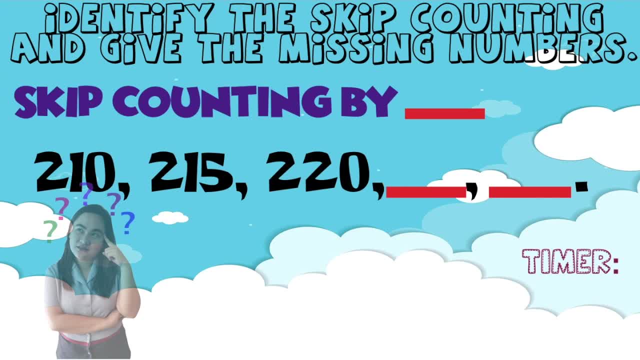 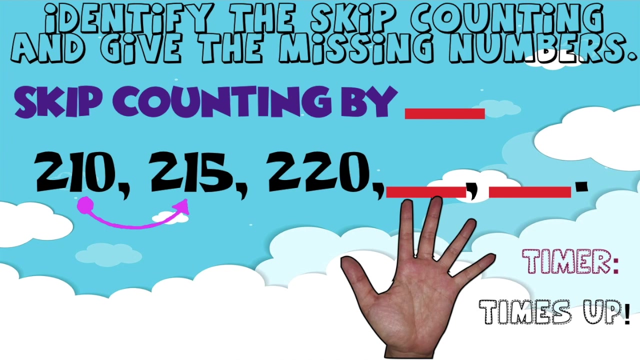 Time's up, Okay, so let's check your answers. So let's count from 210 until we reach 215. 210 in your mind, 210, 211, 212, 213, 214, 215. So that means from 210, 215 is the fifth number. 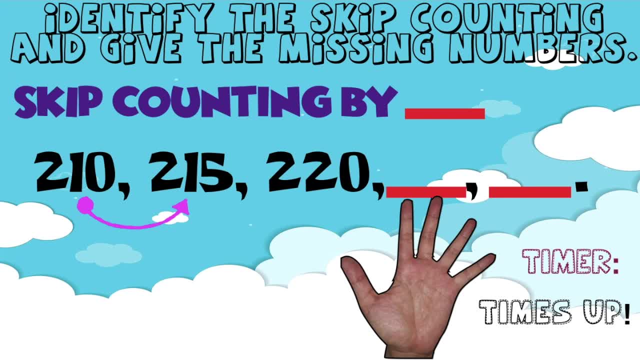 That's why we're going to use keep counting by. That's correct, it's by fives. Okay, so now let's start counting from 220. So 220 in your mind, 221, 215, 222, 223, 224 And 225. Okay, let's have the last one. 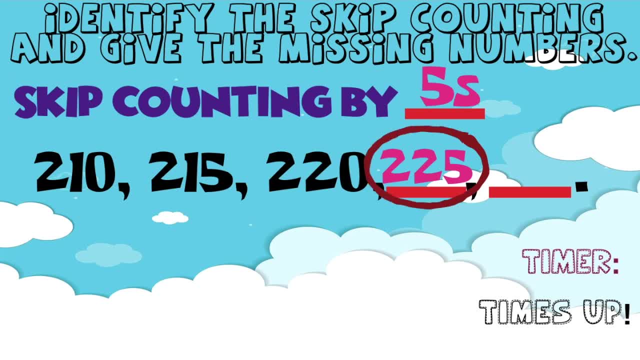 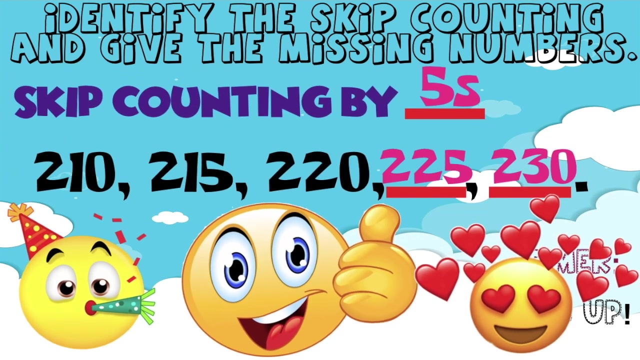 225 on your mind. Okay, let's use your fingers: 225, 226, 227, 228, 229 And 230, 228, 229, 228, 229, 2210, 2211, 2212, 2213, 2214, 2215. 2216, 2217, 2218, 2219, 2219, 2219, 2220, 2221, 2221, 2225, 2226, 2227, 2228, 2229, 2230, 2230, 2240. 2240, 2250, 2275, 2260, 27, 2253, 2295, 2278, 2278, 2278, 2279, 2278, 2289, 2299, 2290, 2290, 2221, 212. 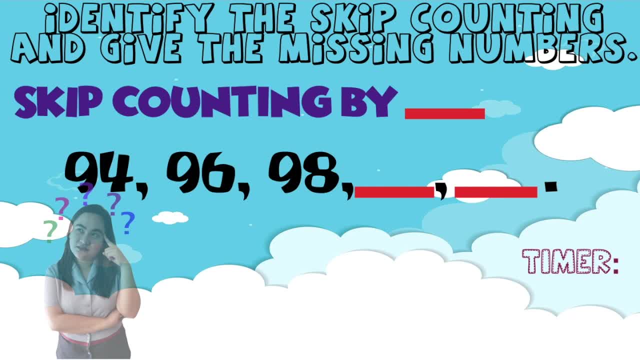 2221, 2222, 2222, 2223, 2221, 222221, 222222, 2223, 2224, 2225, 2225, 2225. So let's see if your answer is correct. So now let's count from 94 until we reach 96 for us to find what kind of skip counting are we going to use. 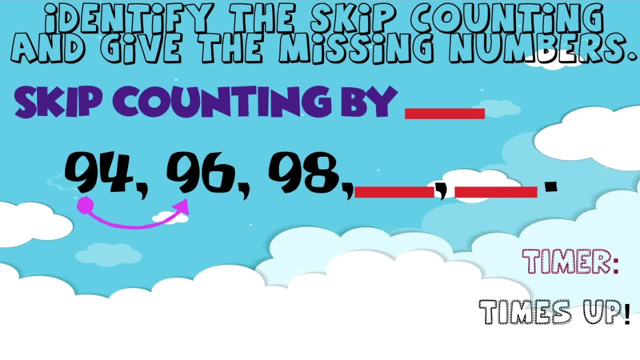 So 94 on your mind, 94, 95, 96.. So we are going to use skip counting by 2s. That's correct. So now we're ready to find the next missing numbers. So let's start at 98.. 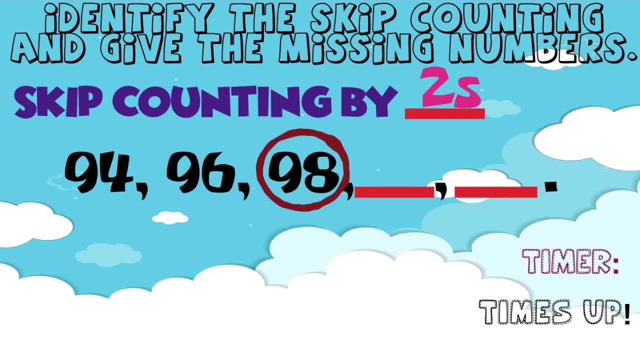 So 98 on your mind, 98,, 99,, 100.. We have 100 here. Let's find the last number: 100 on your mind, 100, 101, 102.. So we have 102 here. 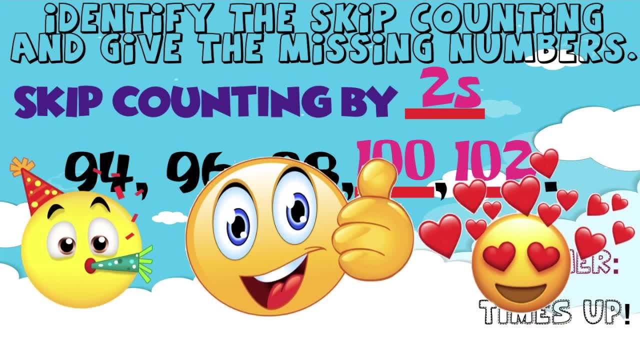 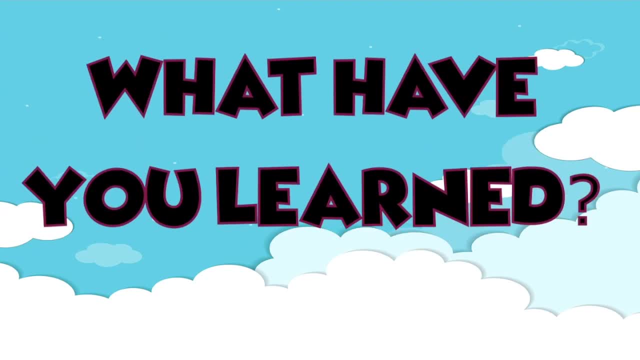 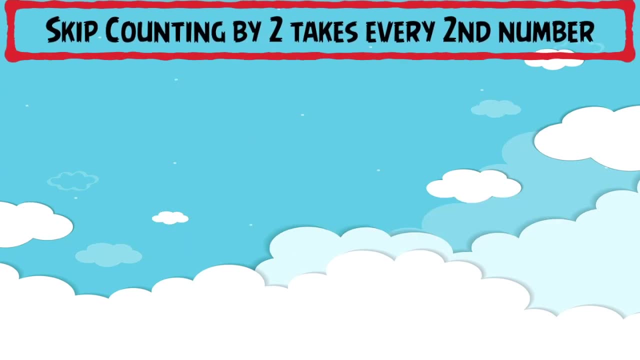 So this is skip counting by 2s. What have you learned? Skip counting by 2s takes every second number. That means if you want to find the next number, you need to add 2 from the number. So skip counting by 3 takes every third number.